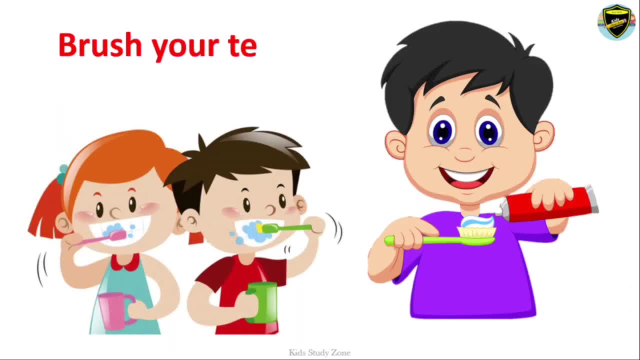 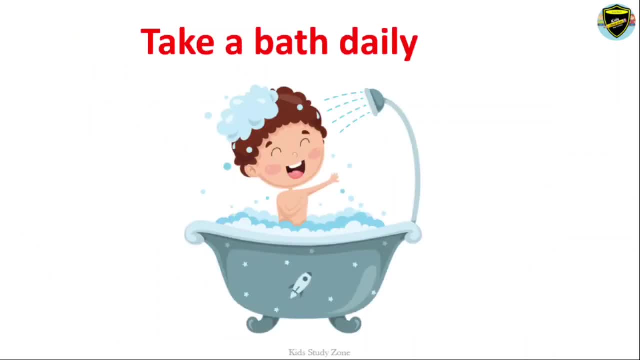 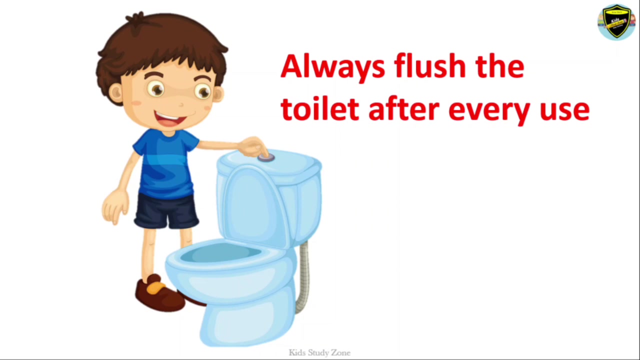 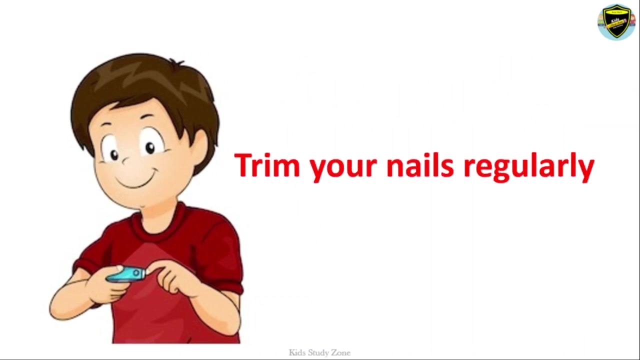 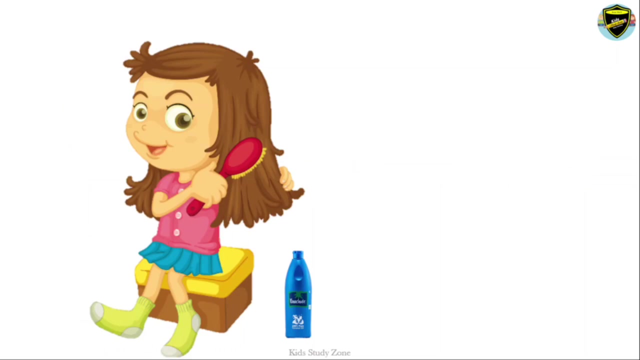 to wake up early. Brush your teeth twice a day. Take a bath daily to keep yourself safe from the germs. Always flush the toilet. Wash your hands before and after every use. Trim your nails regularly- It should not look dirty. Comb and oil your hair regularly. Wash your hands before and after each meal. 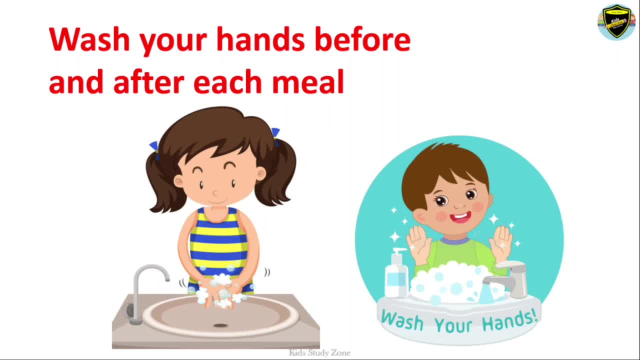 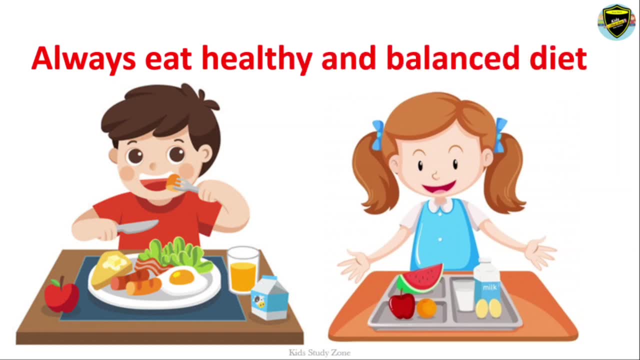 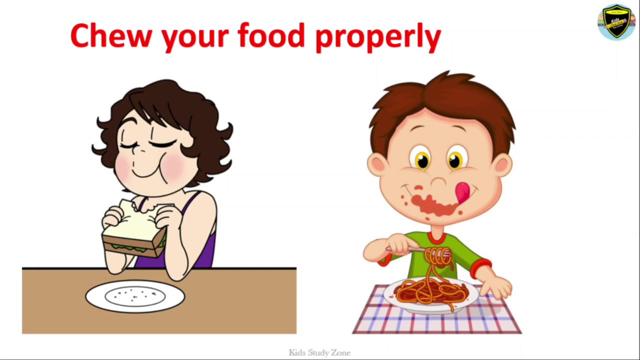 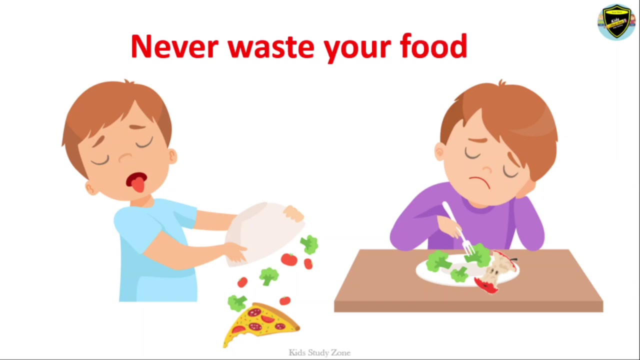 And even after coming from the washroom. Always eat healthy and balanced diet. Add more fruits and green leafy vegetables in your diet. Chew your food properly. You should not eat fast. Never waste your food. Always take the amount which you think you can finish by your own. Never waste the food. 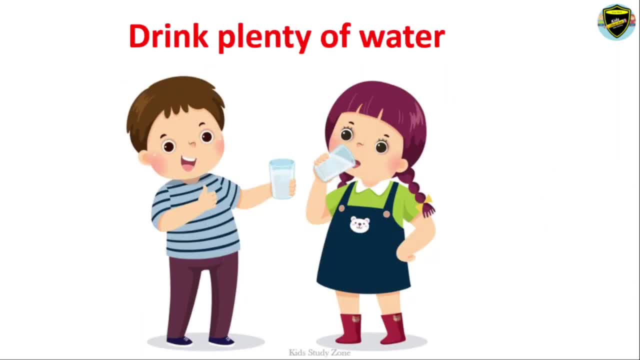 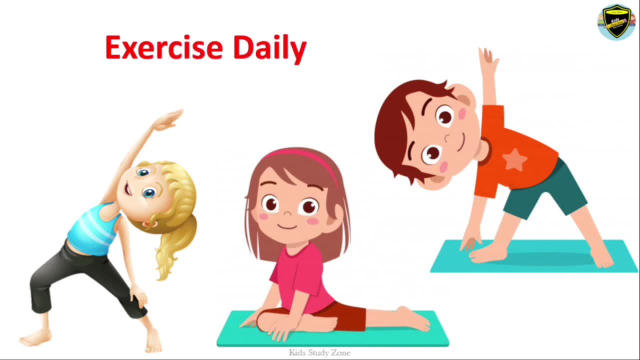 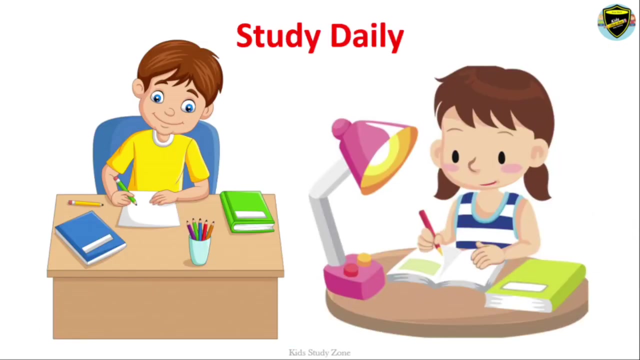 Drink plenty of water. Water is very important for the digestion of the food. Exercise daily. In order to get a fit and active body, we need to exercise daily, And both smoking and drinkingảng and consuming infections will start in your body. 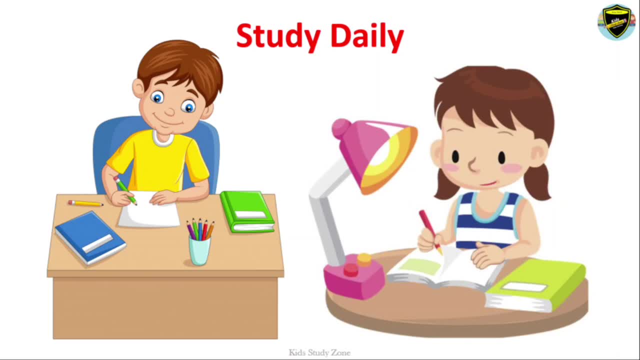 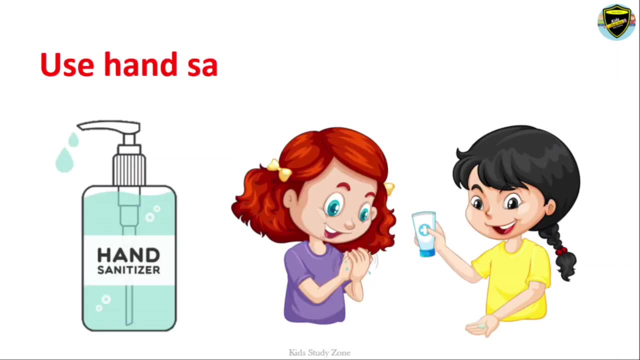 We should stick to our diet in addition to supplements. Which message do you want to give your friends & family to spoons Study daily? We should keep a proper time for the study And we should keep our study table neat and organized always. 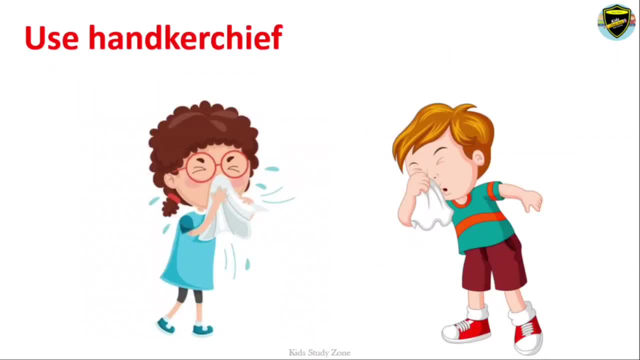 Use hand sanitizers while going out. Used handkerchief while sneezing & coughing. Drink Lyme juice and water. Drink water and water with water. Use handkerchief made of soil. Drink water and water every day. Disinfect your 업 and defeatời repliesЬmsescom. 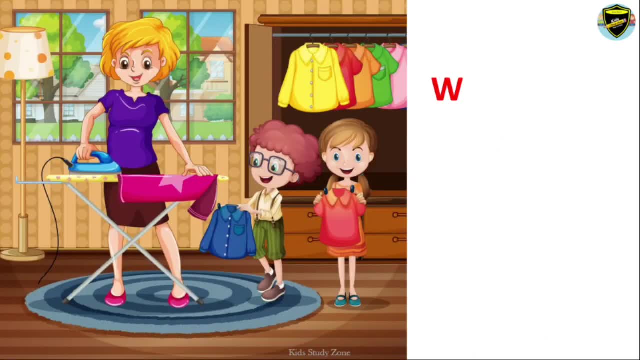 After a nap comes a crews asked to clean your clothes and speed regime may start drugs. You typically get the recommended, but not most of them do so. e-mail to ns umbrella and you can territorially Wear clean and ironed clothes whenever you go out. 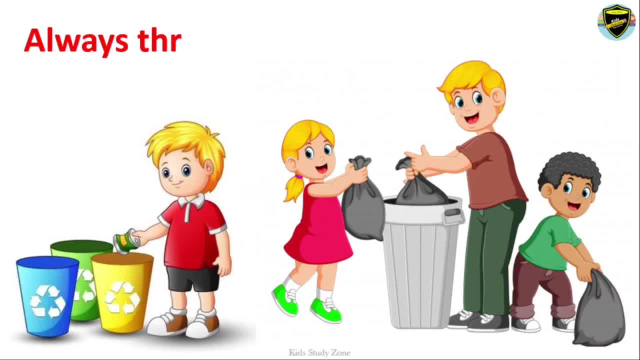 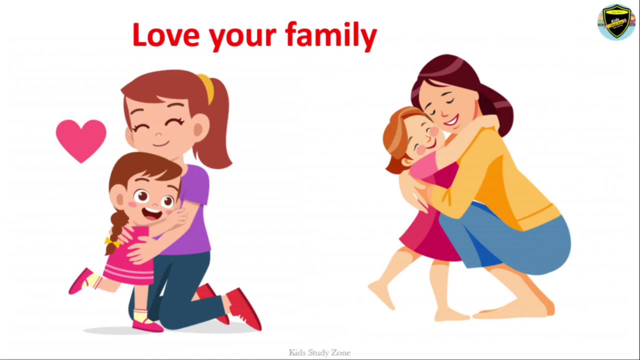 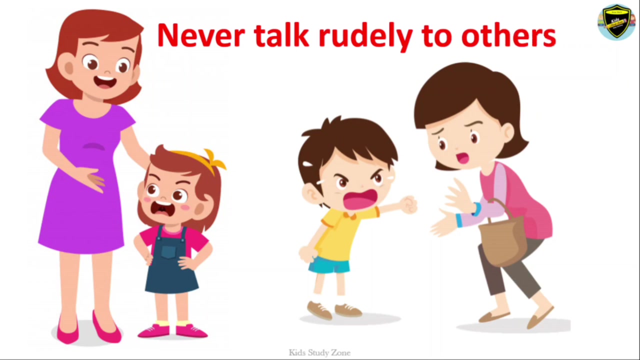 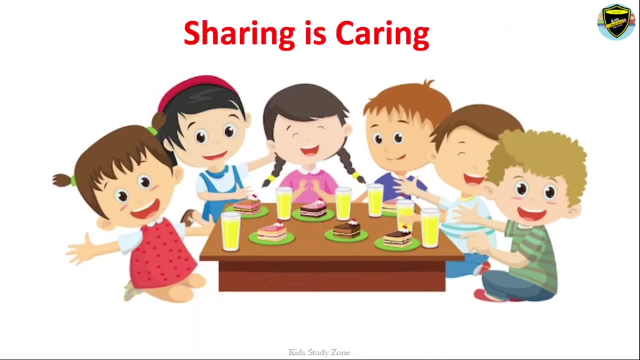 Always throw garbage in dustbin. Keep your surroundings neat and clean. Love your family and be thankful to them always. Never talk rudely to others, especially your parents and your elders. Sharing is caring. We should always share with our friends, as sharing gives us more happiness. Keep your room neat and tidy. 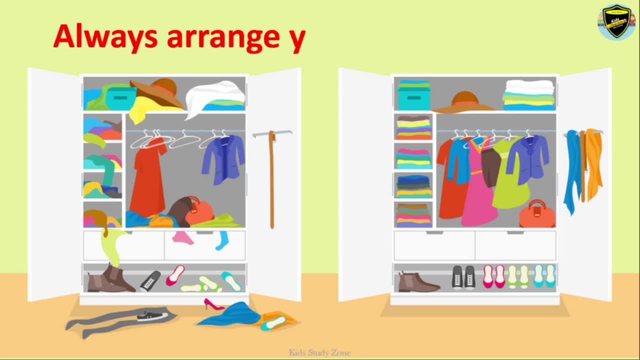 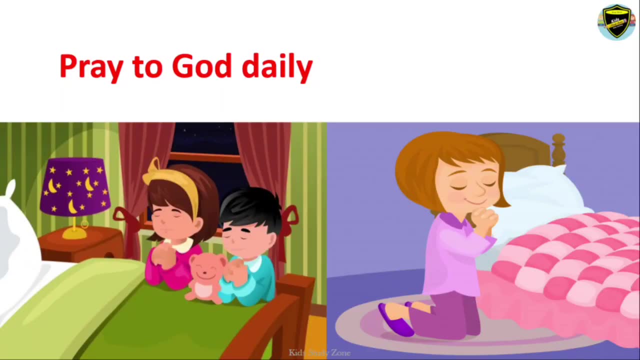 Always throw garbage in dustbin. Always throw garbage in dustbin. Always arrange your cupboard. Pray to God daily. We should always thank God for everything. In the morning, we should thank God for a beautiful day. Before going to bed, we should thank God for keeping us safe throughout the day. 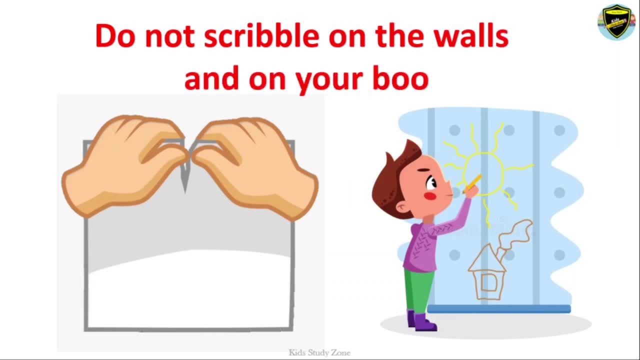 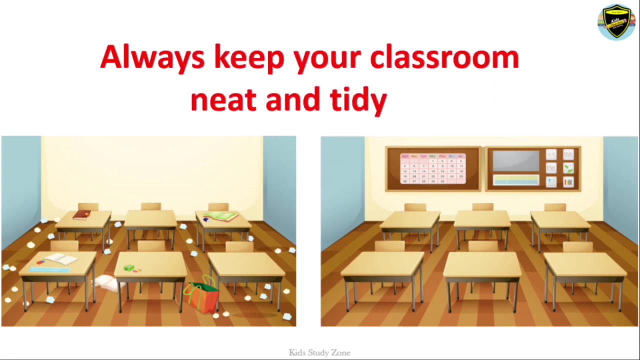 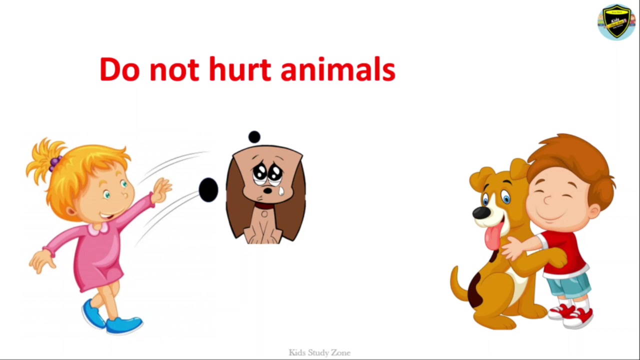 Do not scribble on the walls and on your notebook. Never tear the pages of your books and your notebooks. Always keep your classroom neat and tidy. Don't throw pages and anything here and there. Do not hurt animals. We should always love the animals, as they too need our love. 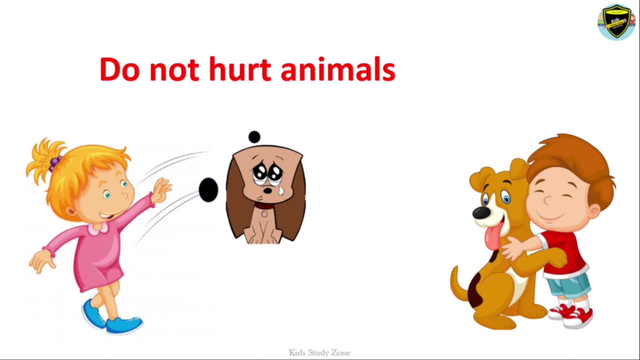 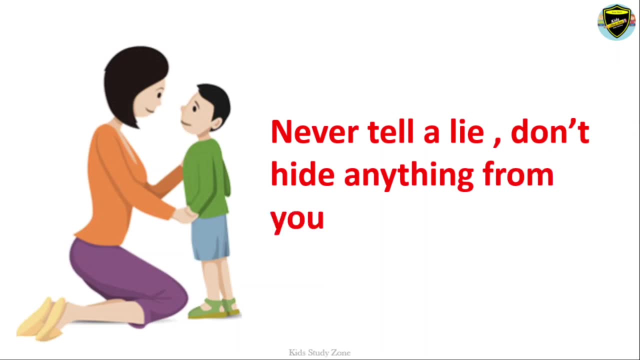 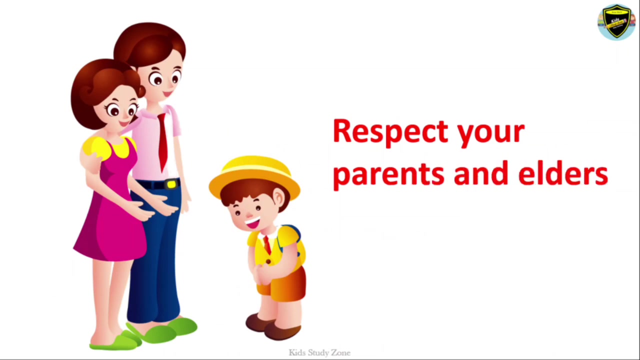 We should never hurt them and we should never throw stones on them. Never tell a lie. Don't hide anything from your parents, As they will love us and they will understand us. Respect your parents and elders. We should always love the animals, as they too need our love. 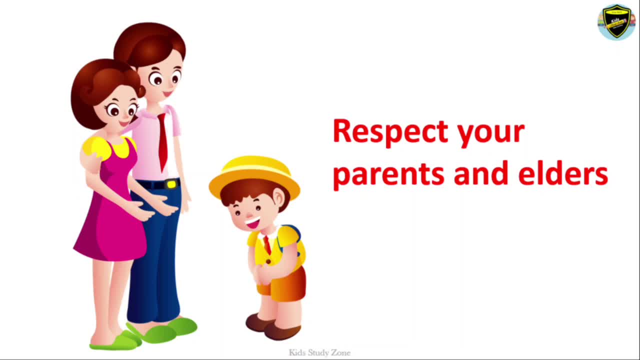 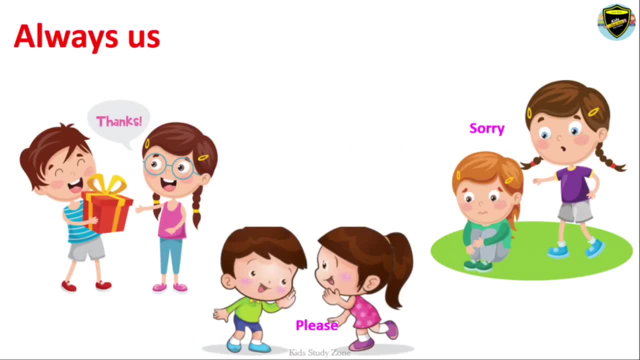 We should always wish them Good morning, good afternoon, good evening and good night. Always use magic words while talking: Thank you when you get something, Please, when you want something, Sorry when you make a mistake. These are the magic words which can bring a lot of happiness around us.